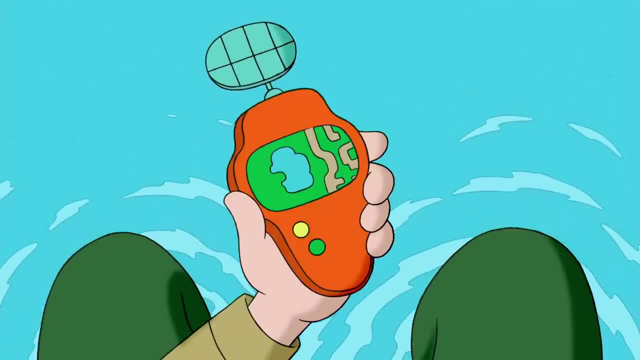 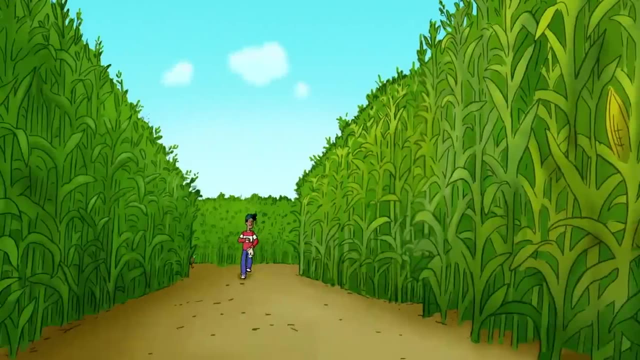 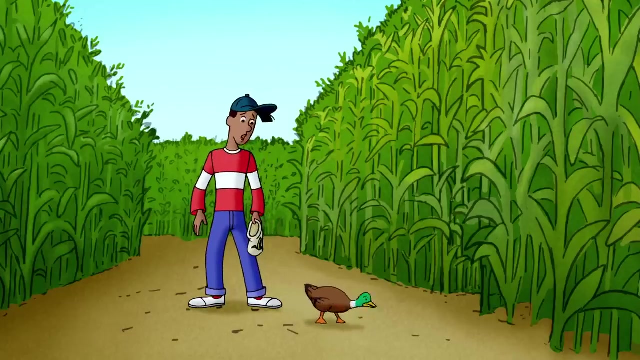 Tina has a solar panel. Why are you sitting in water? I can't leave you alone for a minute. Say what? Hey, No wonder my corn markers aren't here. They're in the belly of a maze-munching mallard. 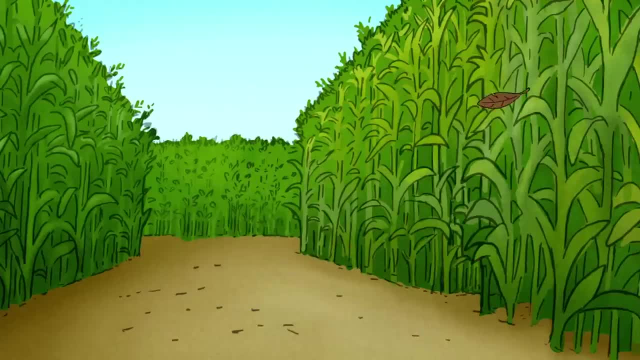 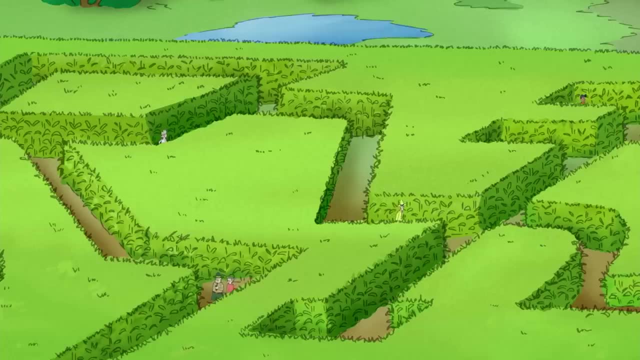 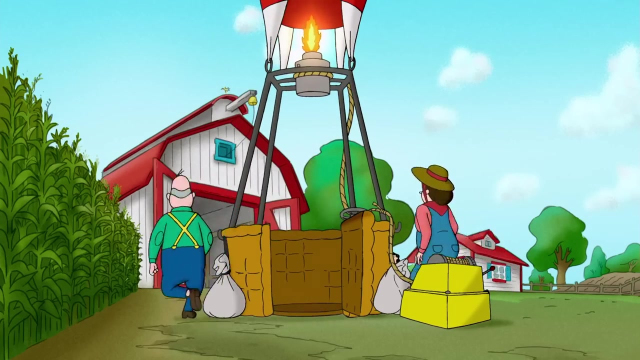 C-cut that out, Do it. What a crazy race. At this point, ladies and gentlemen, anyone could cross the finish line first, And I'll be there when it happens. Where to next, George? We're almost to the finish line. 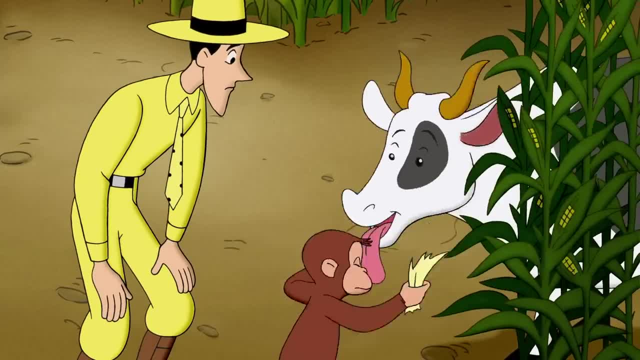 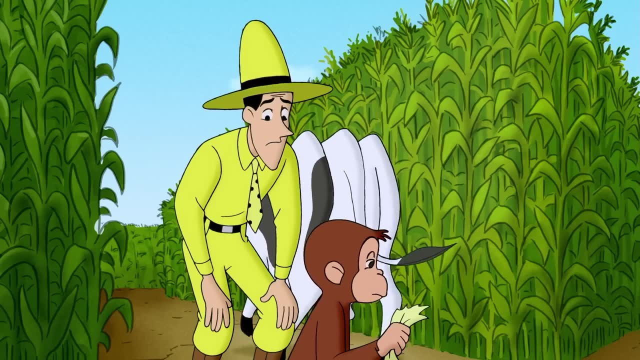 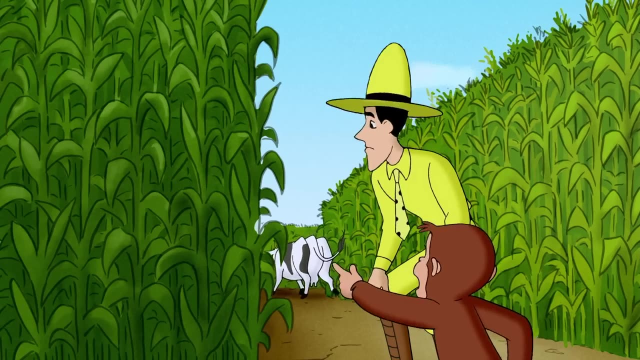 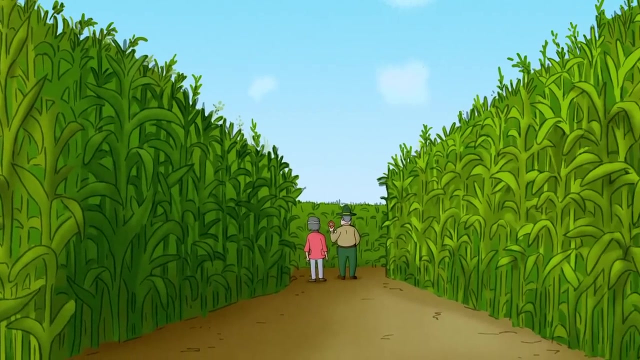 Our map Out of the way. Kel Gee, without a map, what do we do? Follow the cow, Don't you still want to race? Turn left for a shortcut. I hear them, They're coming. It could be all over any second. 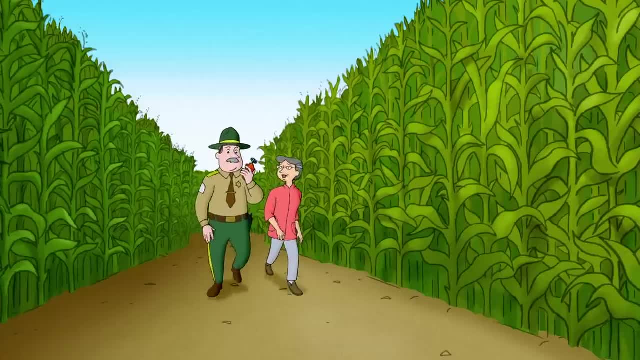 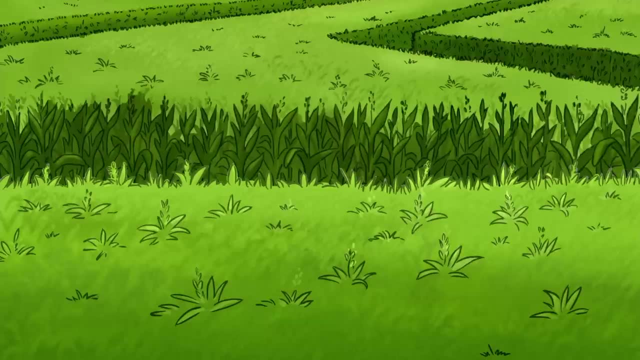 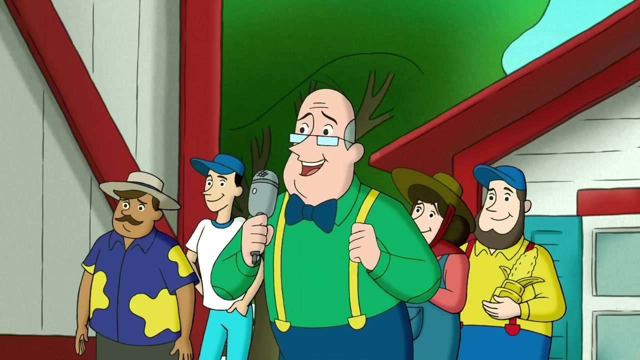 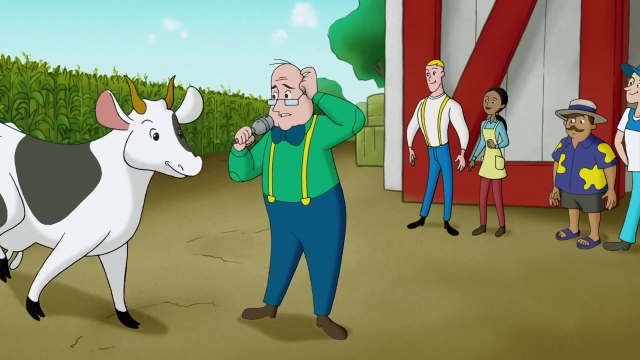 Continue straight. No, stop it. Put it out. Why are we chasing a cow, George Coming through? No, no, no, no, Nope. This is it, And the winner is a cow. A cow, I don't think the cow's a contestant. 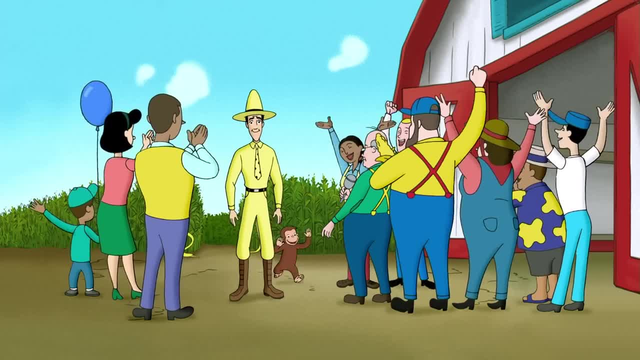 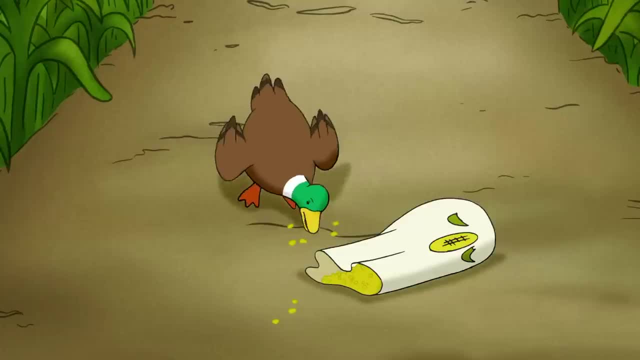 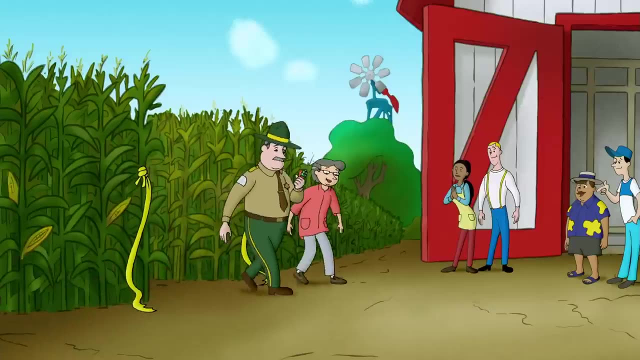 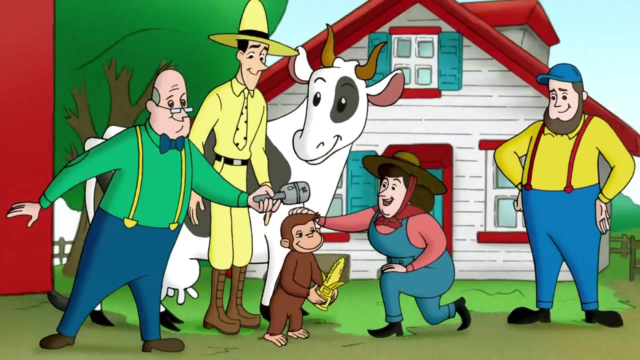 No, this is our winner. Team George, We won Here. I don't need it anymore. Well, makes us third Stop Destination reached. Excuse me, Looks like you two win the Golden Cob. That's one smart monkey. 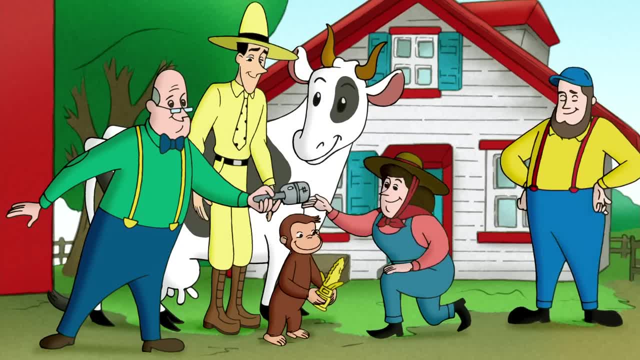 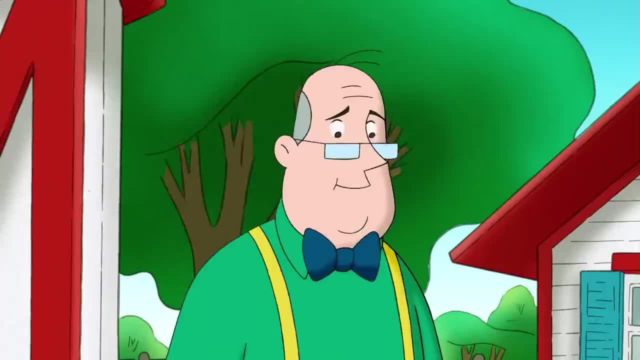 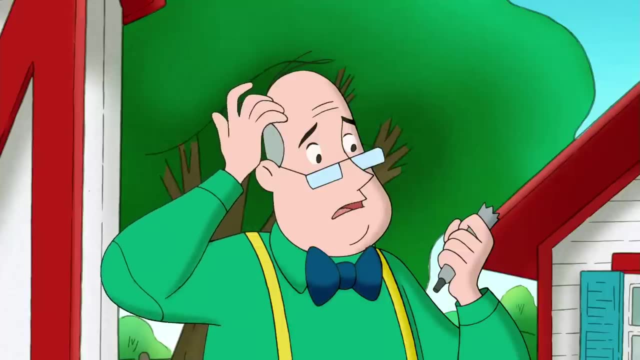 knowing that Leslie can always find the barn at milking time. Oh, very clever, George. Cool trophy race, Uh-huh. Yes, listeners, it has been quite a day. Has anyone seen my microphone?